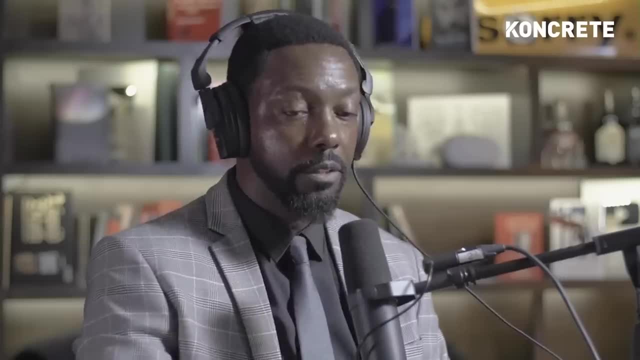 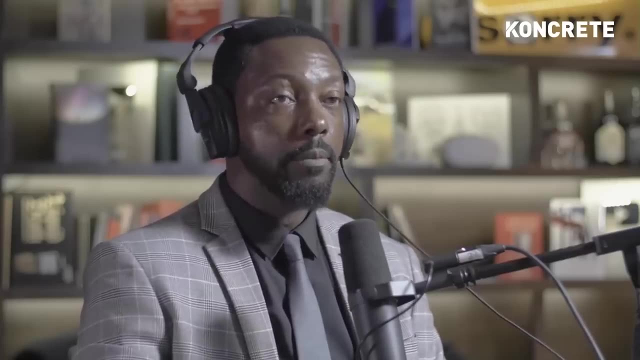 Just as vast as ours is vast, And from higher dimensions, they experience time differently. Time really doesn't exist. The past, present and the future happen all at once, So somebody, for example, from the 50th Imagine would look at us and they'd be able to see us. 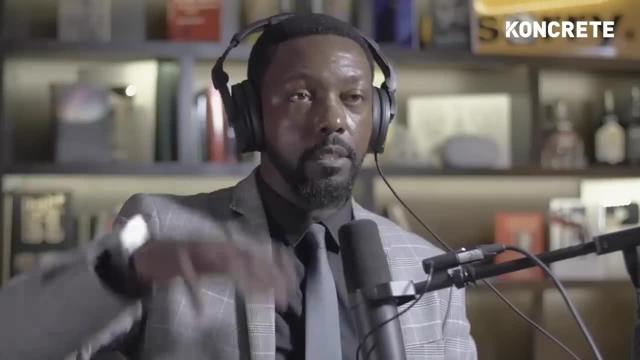 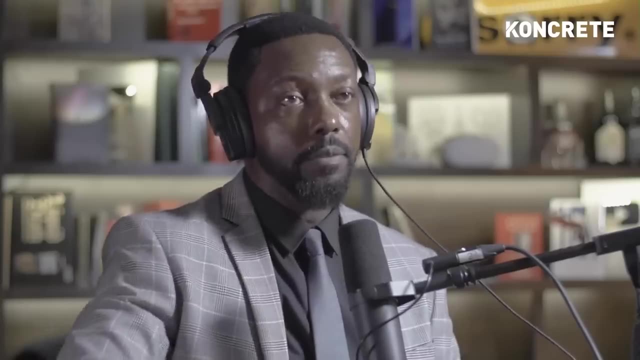 Imagine us in this building here, but imagine when I first walked in and imagine us in here and imagine me like in the bathroom or something. They'd be able to see us in all the different rooms. The different rooms represent different time frames of existence within this structure. 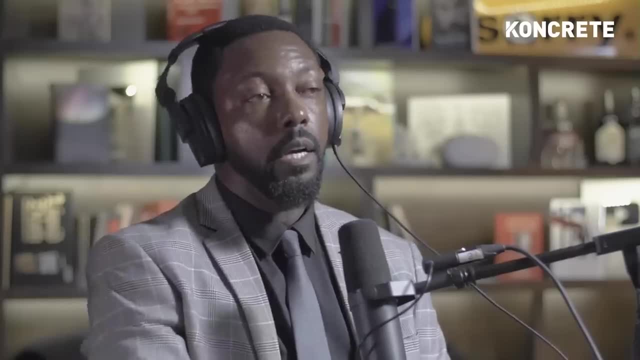 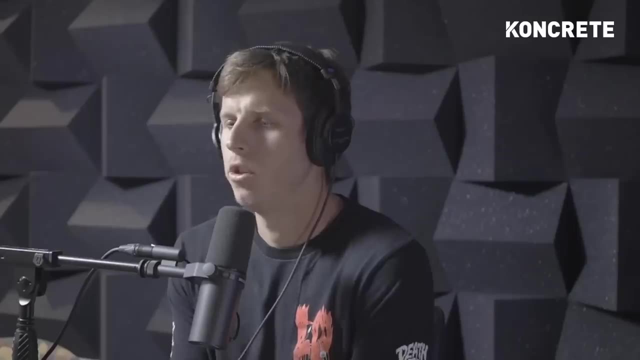 So they could see the past, present and future at the same time. You know, so it's pretty cool. Weird stuff starts happening the higher the dimensions you go. So is the idea that when you're in a higher dimension, you can see below, lower dimensions. 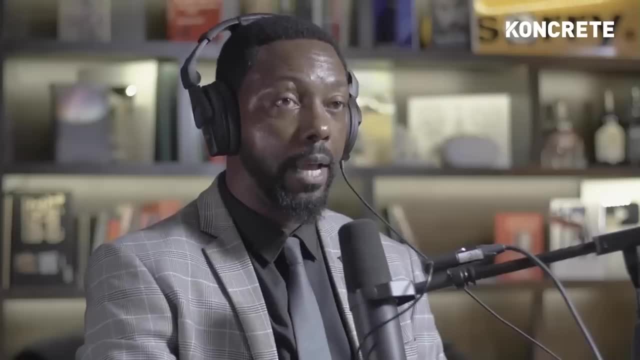 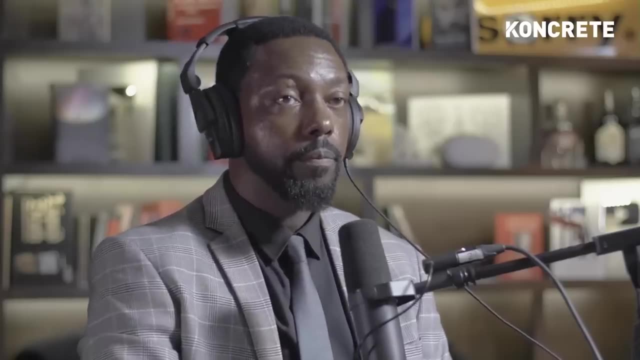 you can't see dimensions above you Exactly, Unless you have the capability of matching. First you have to obtain the frequency of a higher dimension and then match that frequency to be able to walk in. Match the frequency, Yeah, So for example: okay, my hand is stopped now by this table, right. 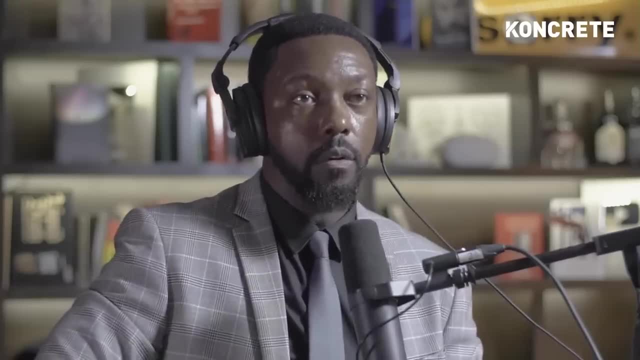 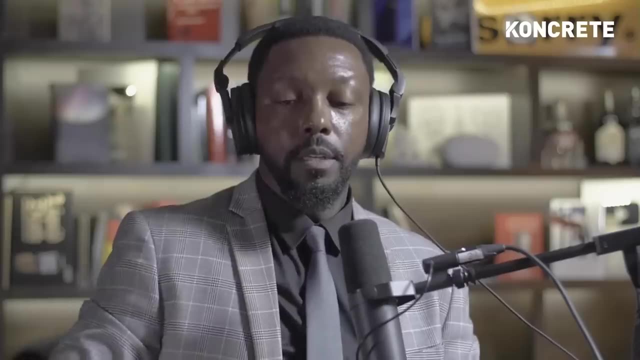 Why is it stopped? I'm not really touching the table. There's repulsion going on. Electromagnetic repulsion between the electrons in my hand is repelling the electrons in the table. You don't really touch anything. Now, if I can match the subatomic frequency of the atom, 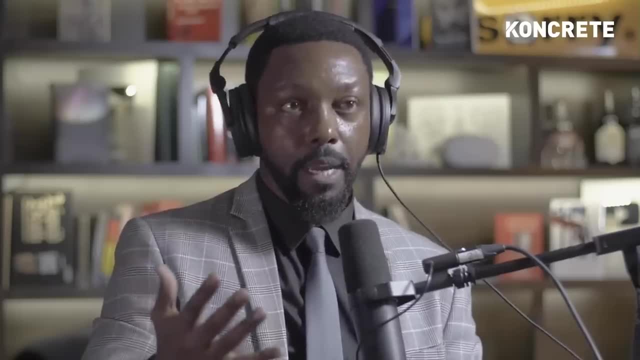 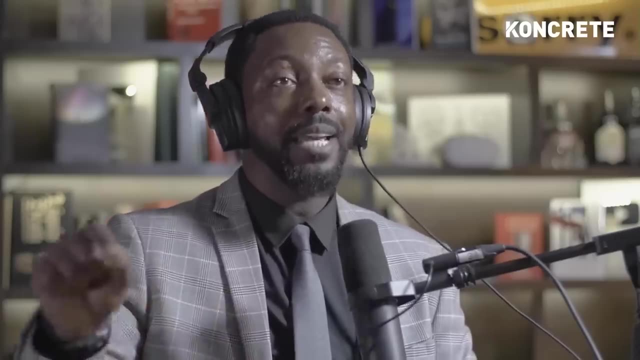 in this chunk of wood here on this table, with my hand. I would be able to pass my hand right through this table unscathed. Why? Because atoms are 99.999% empty space. Nothing is really here. Everything is only a light wave slowed down to a particular frequency. 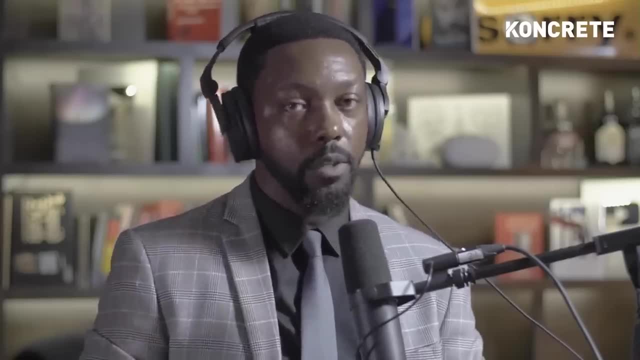 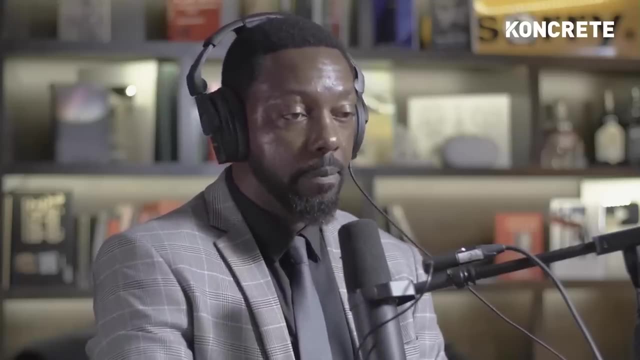 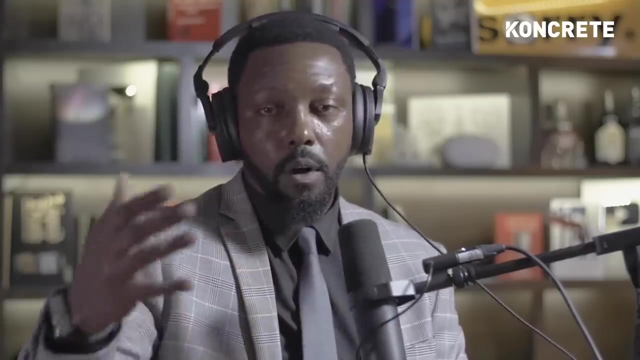 And so if you can match frequencies, you can merge with things, You can walk through walls and all that kind of stuff. The things that seem paranormal could be advanced beings have tapped into some type of understanding of how to match different frequencies in our dimension and appear apparitional or paranormal. 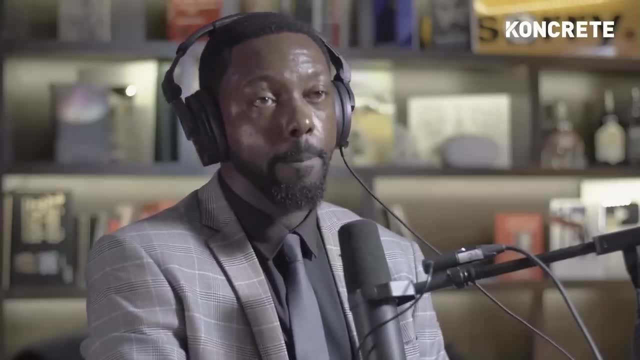 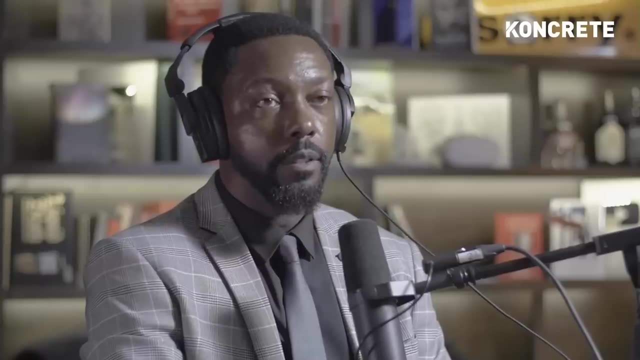 But in true reality they could just be taking a peek in. And how do we come to the understanding that these higher dimensions exist? Like what is the most basic evidence that we have of this? Quantum physics proves it. See, when we look into the quantum world, everything changed. 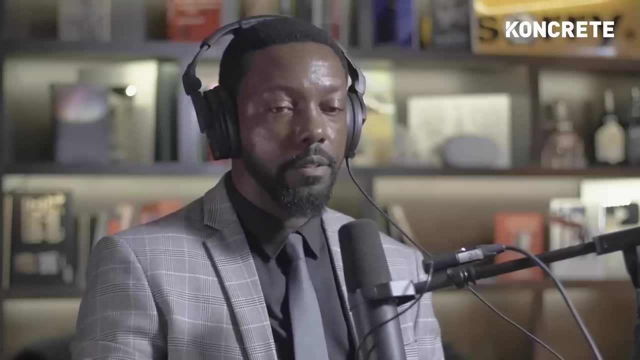 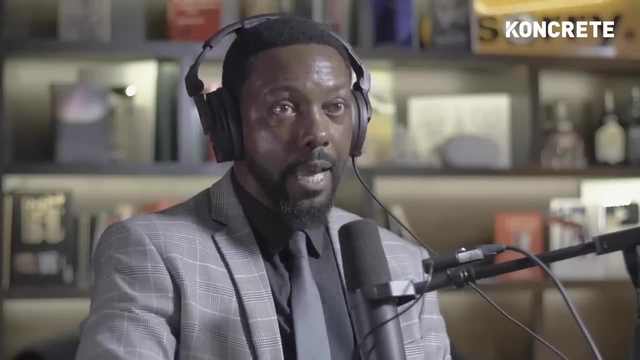 In standard physics is where we are right now in the large side of physics, But the smaller you go, the more weird things get. We find that We find that particles transphase in and out of existence and they go to different dimensions. 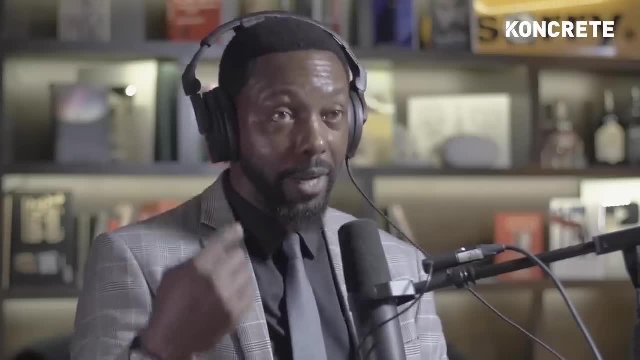 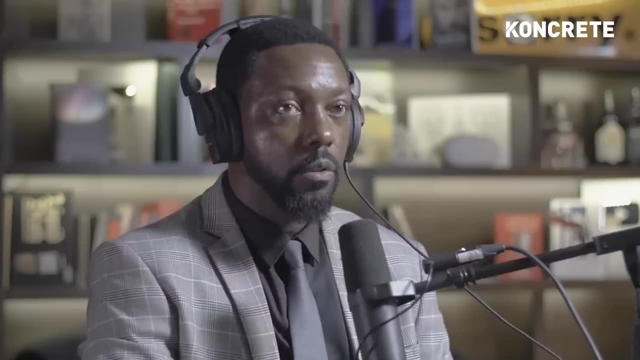 We even know now that some of our synapses of our thoughts in our brain phase out of this dimension and they go somewhere else and then they come back again. And this has all been tracked and traced through the understanding of quantum mechanics and quantum physics. 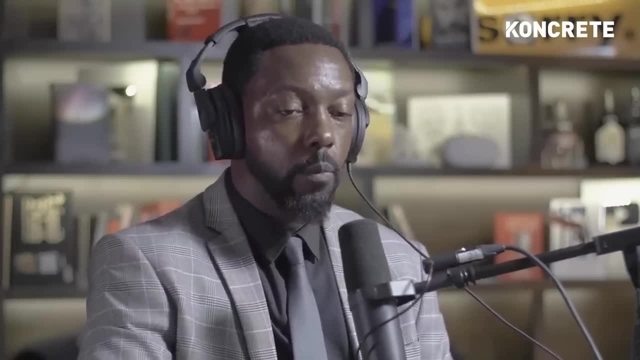 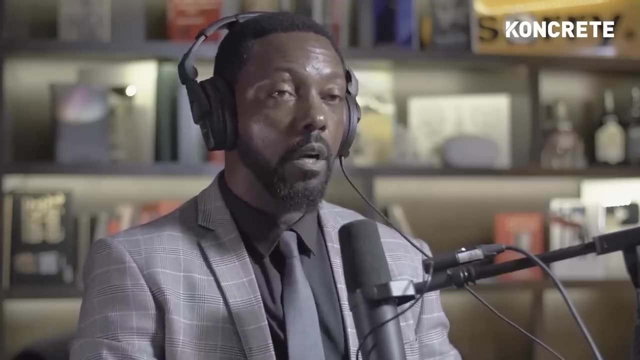 and understanding that dimensions exist. The biggest way that we made a model of this is we figured out how to create something called quasi-crystals. Now, these quasi-crystals are these Multidimensional crystals. We actually created an eighth-dimensional quasi-crystal. 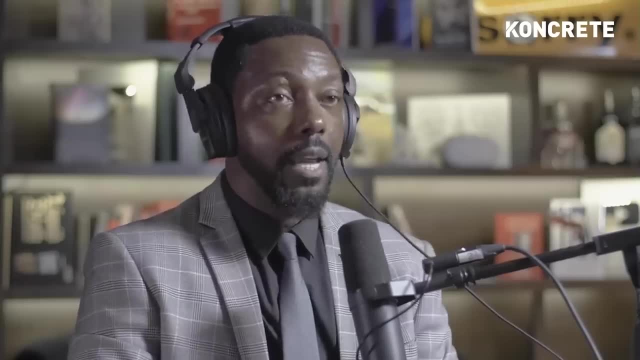 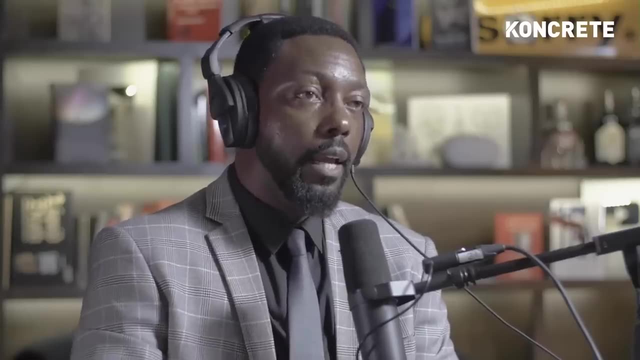 We created this? Yes, we created it. How did we create it? We created it in a laboratory using different technologies, And then, from that eighth-dimensional quasi-crystal it casts a shadow of itself down to a fourth-dimensional quasi-crystal. 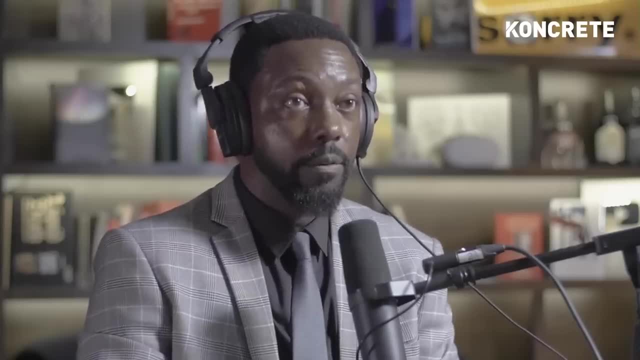 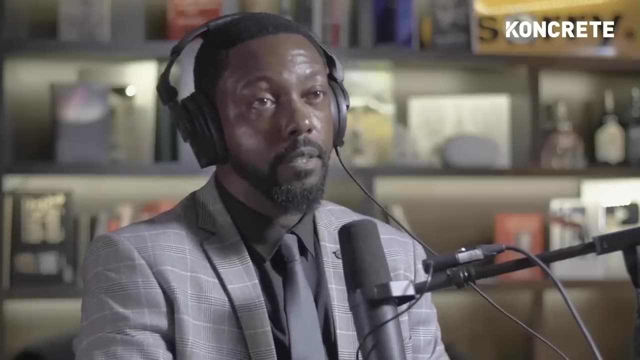 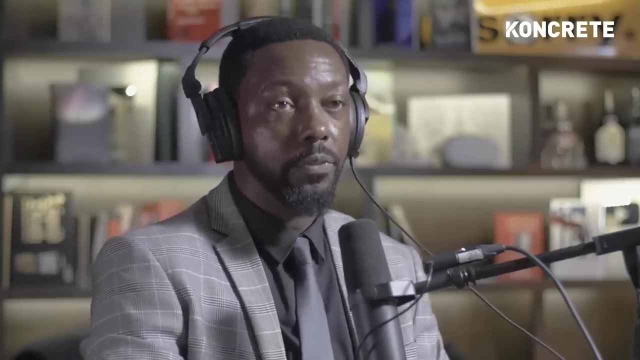 which then casts down a shadow which creates a sphere. So we know that the universe is most likely the shadow of a higher dimension. It's crazy stuff. Yeah, that's kind of mind-bending. We're living in a light matrix which is actually a light matrix, which is a shadow of a much higher dimension. 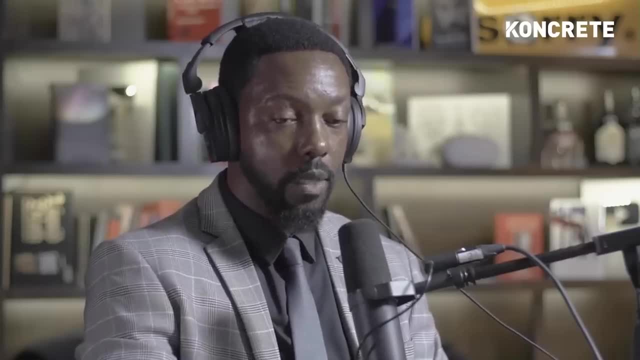 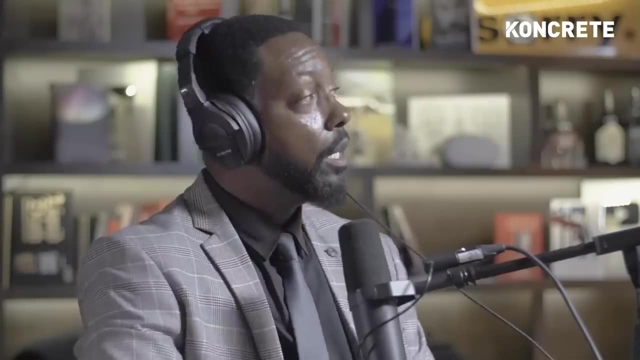 And so we know this, because they created these crystals, these quasi-crystals, and when they put them at different angles, they cast shadows sometimes. What do these crystals look like? You look up the quasi-crystals? yeah, They look like. 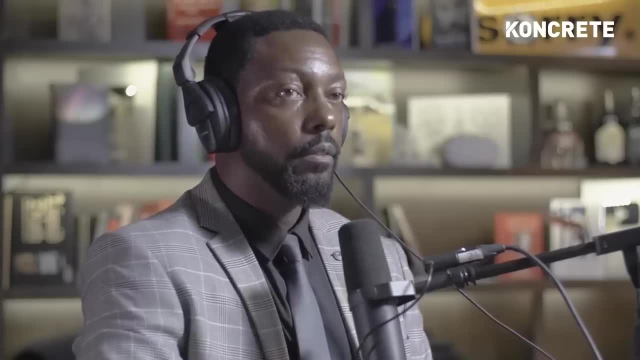 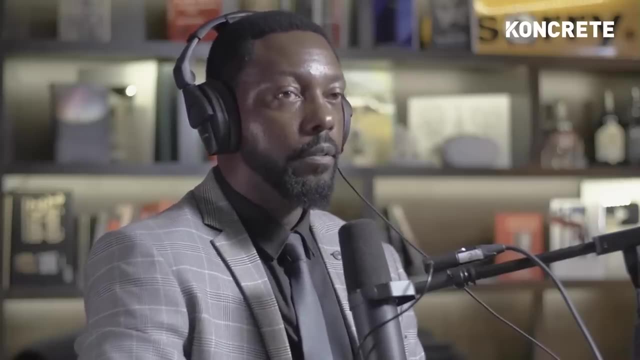 Have you ever seen a Dinkra codes? A Dinkra's? I think I've heard you talk about this before. They look like a Dinkra's. the symbols- mathematical symbols, but in the third-dimensional time-space. And so if you take them and pull them out into a three-dimensional time-space, 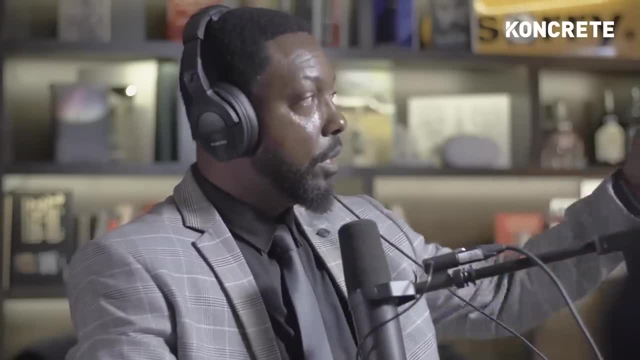 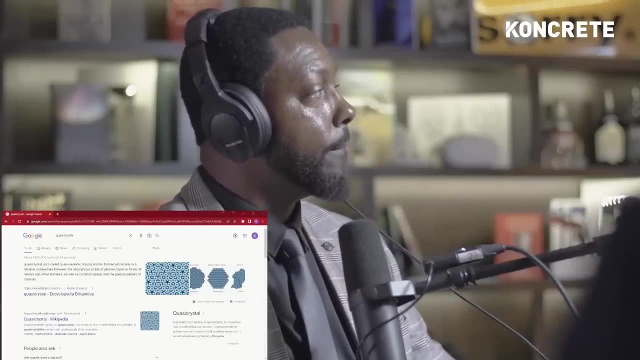 they look like these lines that are connected with these nodes, like that you see Quasi-crystals. This is a quasi-crystal, Yeah, And so It's an ordered structure, but it's not periodic And it's got a crystalline pattern. 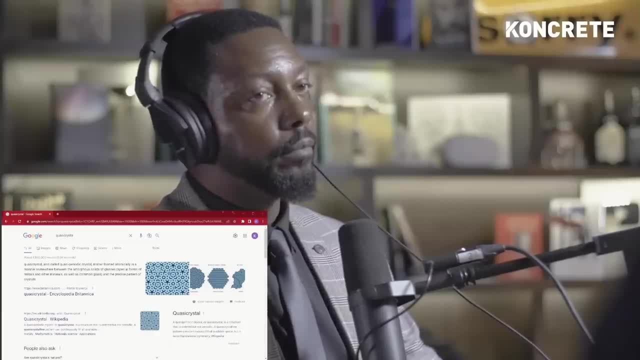 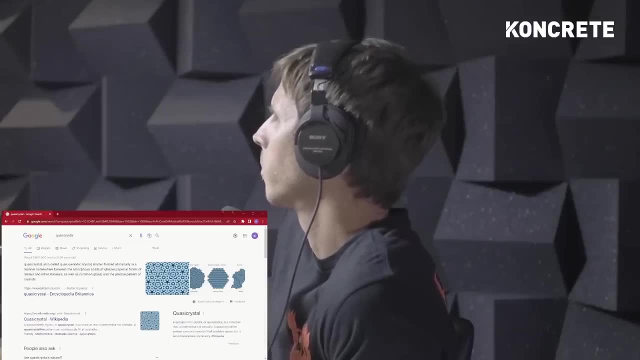 It's formed atomically in a manner somewhere between the amorpha solids of glasses, special forms of metals and other minerals, as well as common glass, and the precise pattern of crystals. Yeah, If you put eighth-dimensional quasi-crystal, you should see some research that comes up on that. 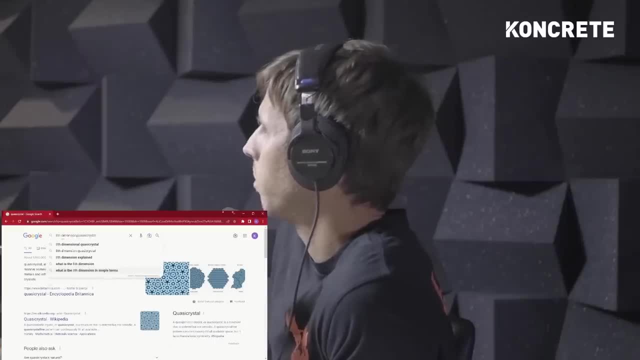 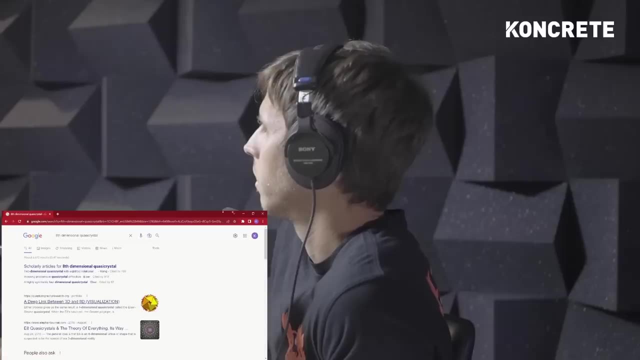 It looks like What you look into: a collider, A kaleidoscope. It's a fractal. It's all about fractal. We live in a fractal holographic universe. The quasi-crystal is a fundamental basis of the fractal holography that we're living in. 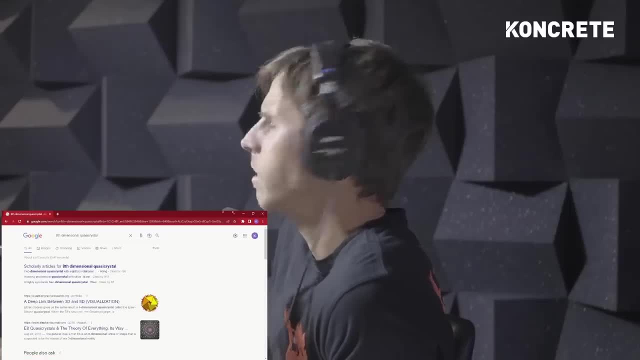 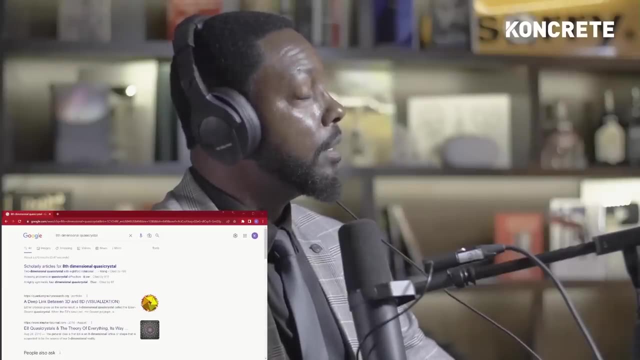 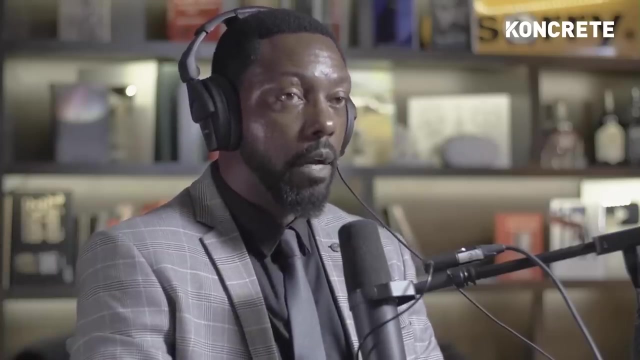 We're fully immersed in it so we can't detect it, but we're living in a light matrix And that's what the Dinkra codes also prove. Okay, Explain the Dinkra codes. What is that exactly? So, Professor James Gates Jr, University of Maryland, former scientific advisor to President Obama, 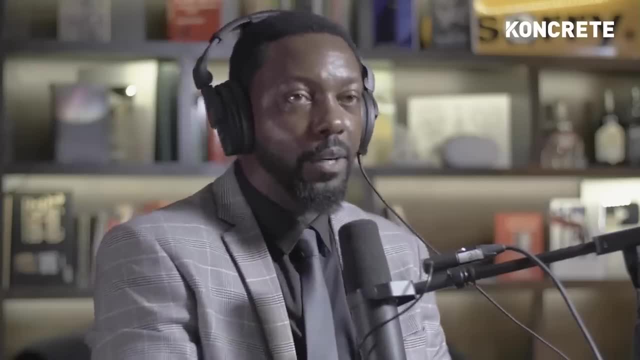 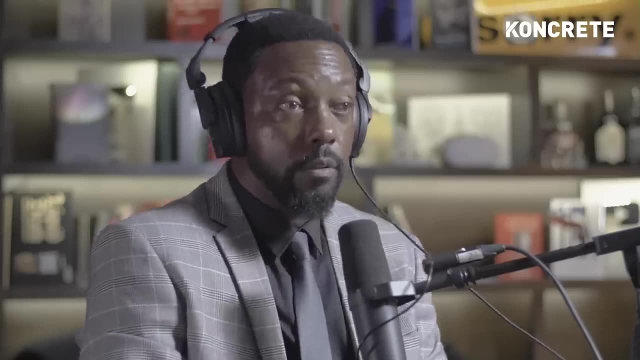 just to give you this guy. He's not just like a jackpot, He's a jackpot, He's like a real dude, you know, Yeah, And he put together a team of the most incredible supersymmetry and theoretical physicists in the world. 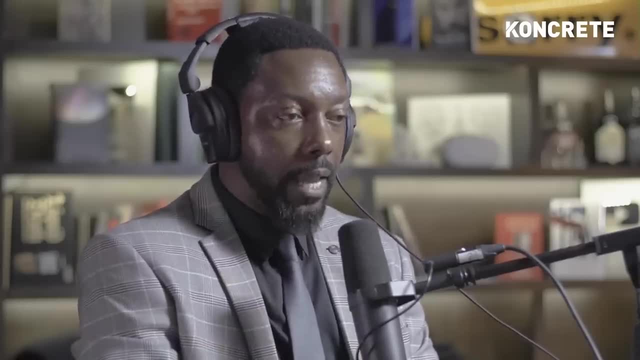 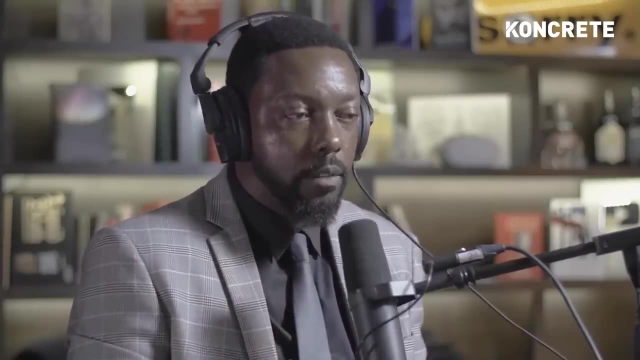 like the top brains in the world on this, And they started analyzing: what is the ether of space-time? What is this soup that we're living in, that we're inhabiting this universe? What is it? What is it made of? What's powering it? 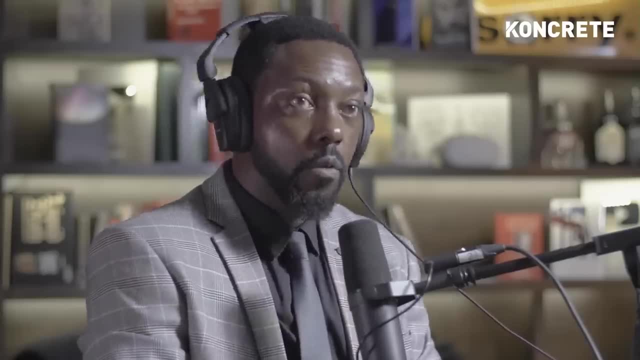 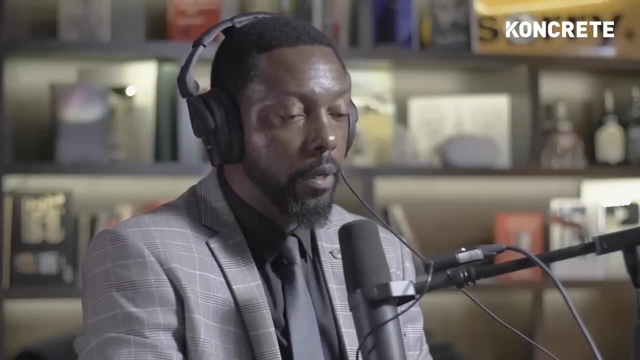 They discovered something called a Dinkra codes, which go back to the ancient Dogon tribe from Mali, Africa. The original inhabitants of the land of Camden moved to Mali later after they were thrown, thrown out, taken over at one point, But they still kept this ancient knowledge in Mali about these Dinkra codes and they would draw these patterns. 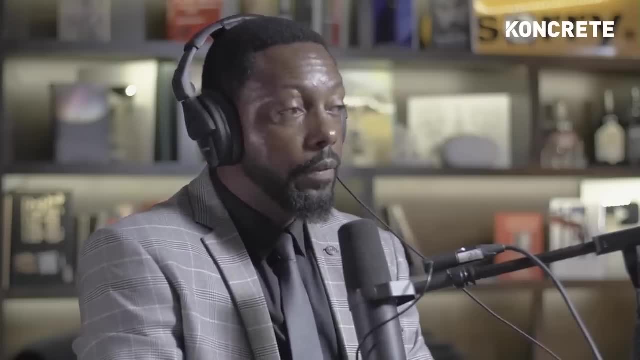 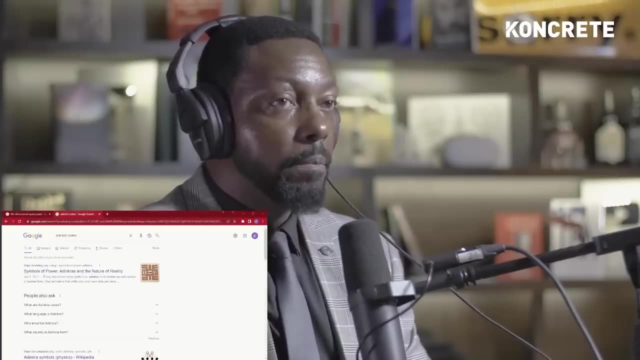 Well, he discovered that these patterns are actually mathematical codes. And these are not just any mathematical code. There goes one there. They're actually the codes that describe the ether of space-time itself. They're error-correcting codes, the same exact codes that run our search engines and web browsers. 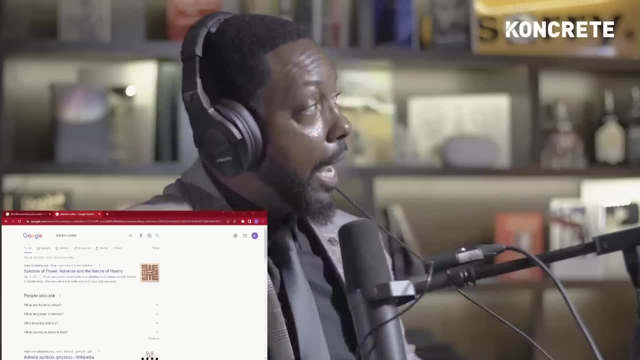 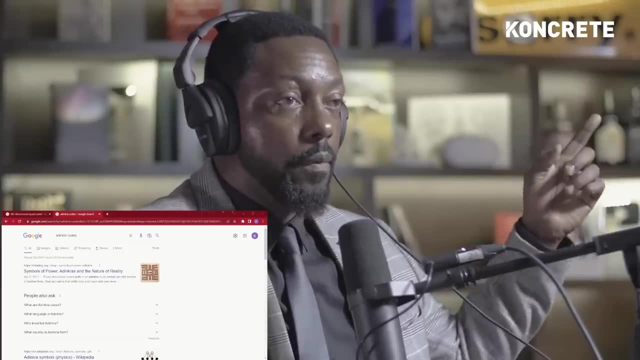 that we're using right now. to look at the image, There's coding behind that screen That runs this, what we just did, and guess what? It's the same code that runs the universe. So we discovered that we're living in a 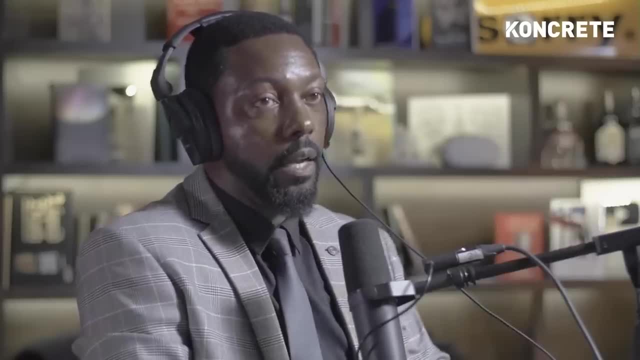 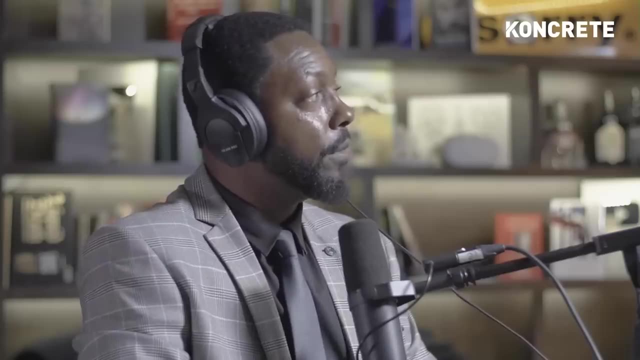 that we're living in a programmed light matrix. There's a software programmer that has written this code. Austin, pull up more images of this. There's all different types of images There you go See. now that You see that one there. 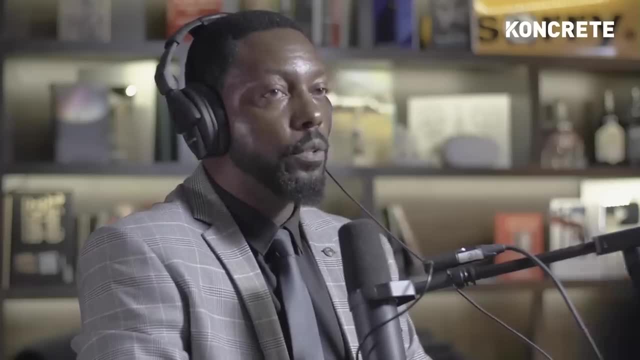 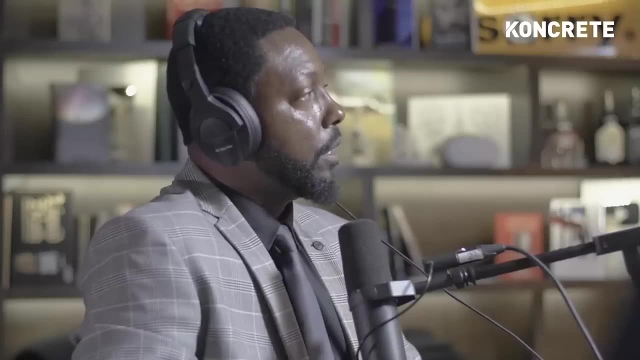 Right there, That's a quasi. That looks like a lot like a quasi-crystal. If you were to shrink it down and put a whole bunch of them in one location, it looks very similar to a quasi-crystal. So these are Dinkler codes and you can see the colorful one that was up there. 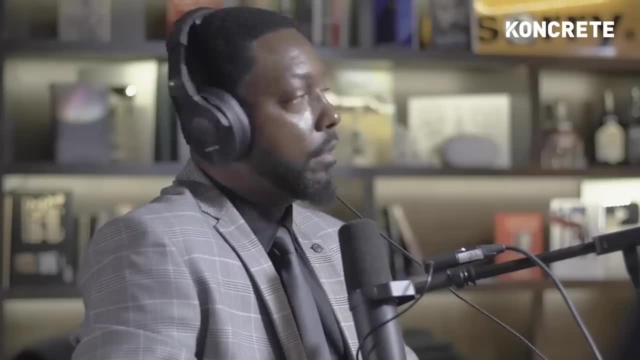 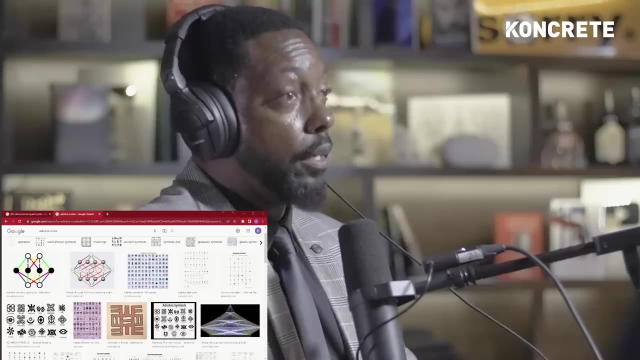 These are depicting the nature of reality. Wow, And they actually are mathematical programming codes. They're a special type of code, though They're error-correcting codes the same type that Google browser is running on. It's the same thing that runs the universe. 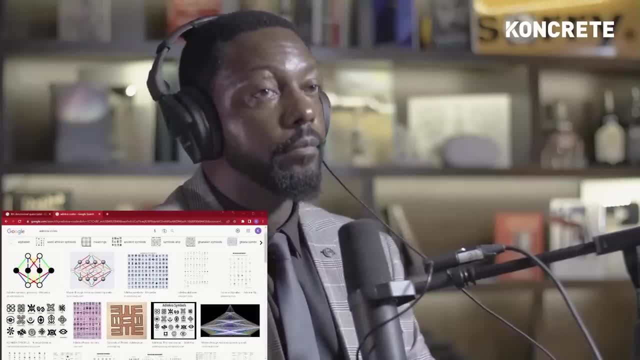 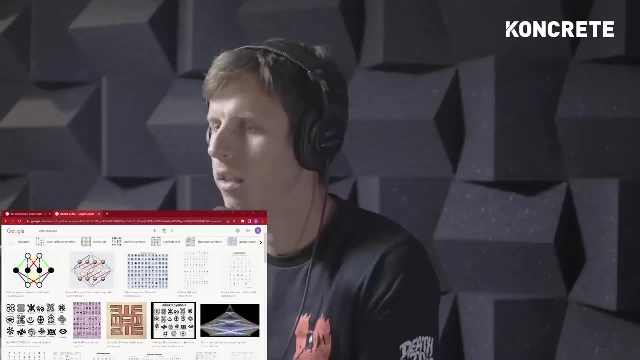 Error-correcting codes. Yeah, And what do we gain from all of this knowledge? What does this tell us? Where do we take this? What is the? Obviously? this is foundational knowledge for us, but where do you see it going? 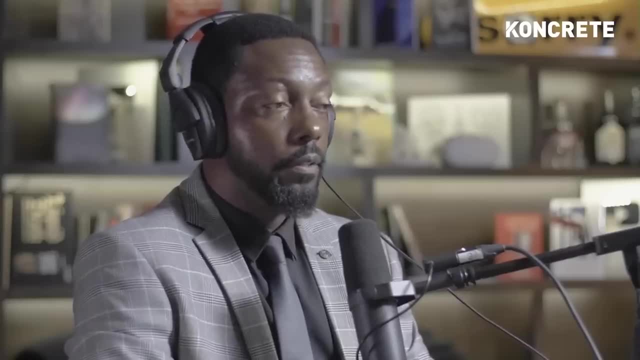 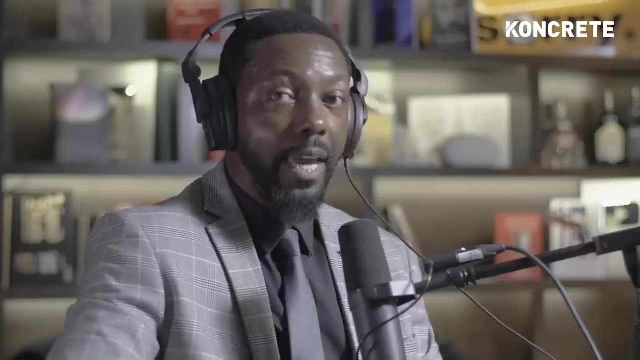 Well, if you understand that we're living in a fractal, holographic light matrix, it doesn't mean we're not real. It just means that there is a creator or creators that were living in, something that was created, just like the ancient texts and all the scribes and biblical texts and everything else says. 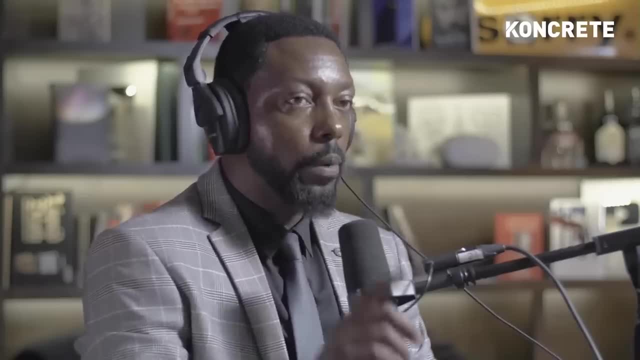 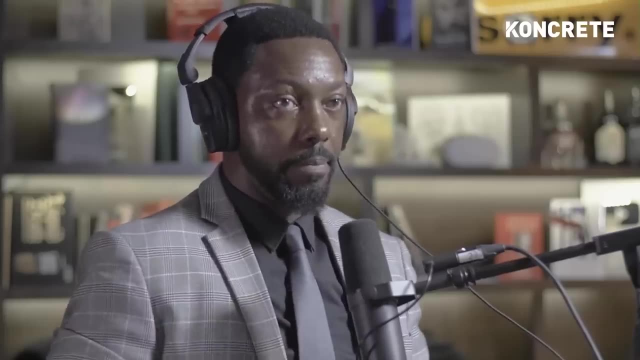 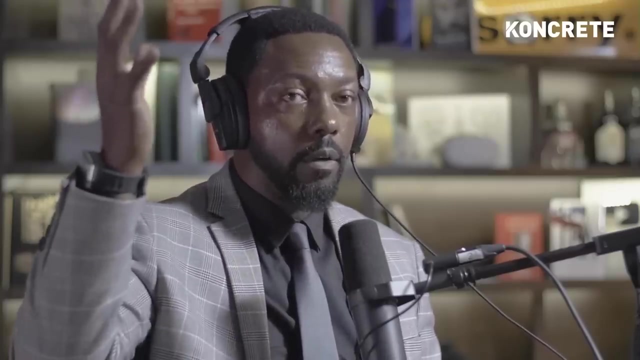 But it tells us: wow, this is the method of the creation. Now we're getting closer to understanding what we really are. We understand now that consciousness isn't made inside this avatar body, that the avatar body doesn't even exist, That consciousness is a stream of something coming from somewhere else. 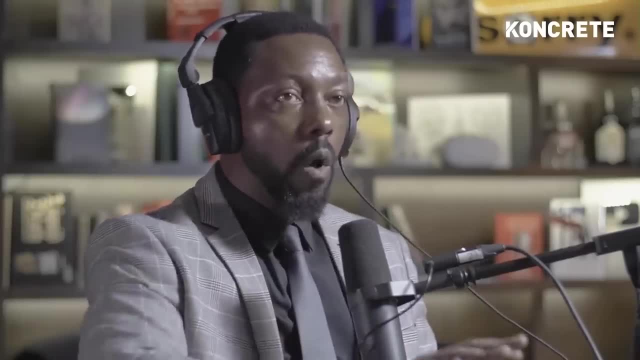 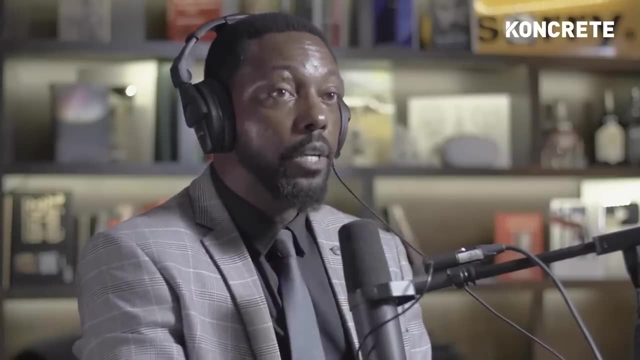 and it's being picked up in this matrix. with this coding: If you took all the humans on Earth, there's eight billion humans on Earth. If I took all eight billion humans and removed the empty space between their atoms, I can fit every human into a sugar cube. 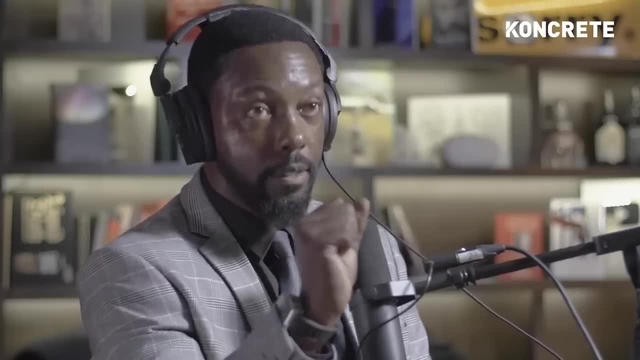 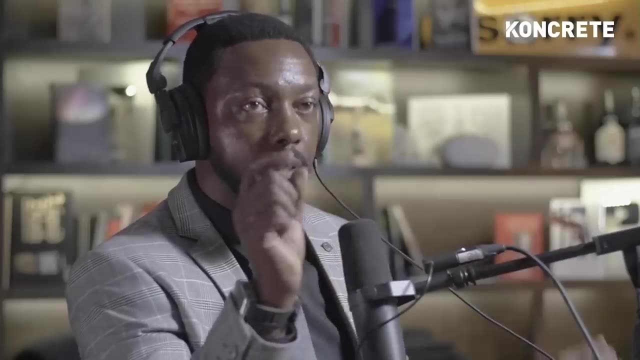 One sugar cube can hold all eight billion of us. Really, Yeah, All eight. All the atoms of eight billion humans, All eight billion people on Earth. See, atoms are empty space. If you take the empty space out, you collapse it into one sugar cube. 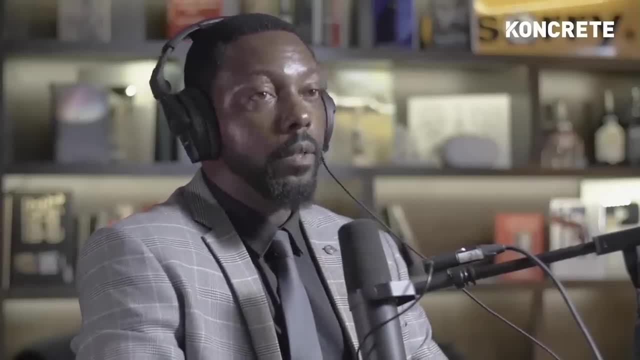 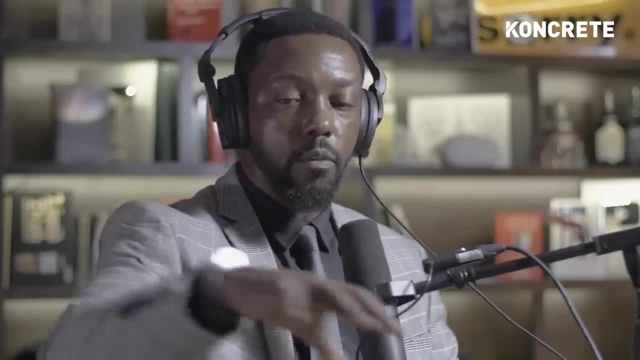 All eight billion can fit in one sugar cube. So what does that mean? That's wild. What's here? There's only one consciousness, it seems, and it's like a radio station that's transmitting out a frequency from a higher dimension. 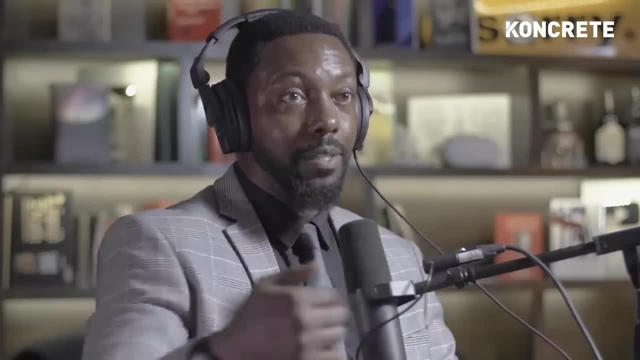 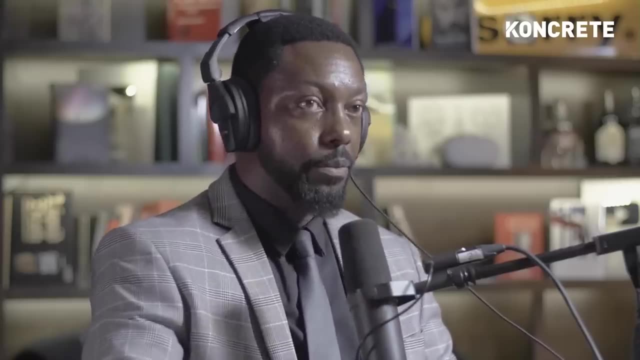 Our avatar bodies pick up that frequency. You're 99.1,, I'm 99.2,, he's 99.3, but it's still coming from the same source, And so we're all coming from the same source. It's like the universe has found a way to live subjectively through multiple entities.